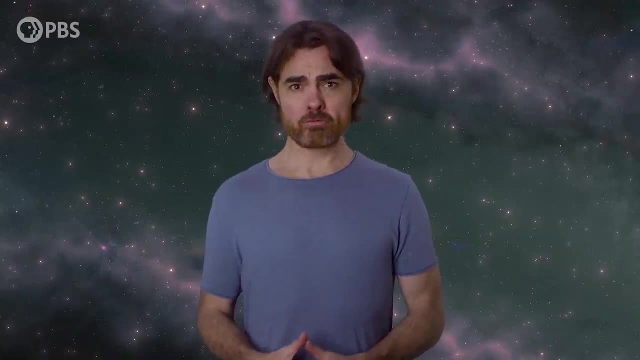 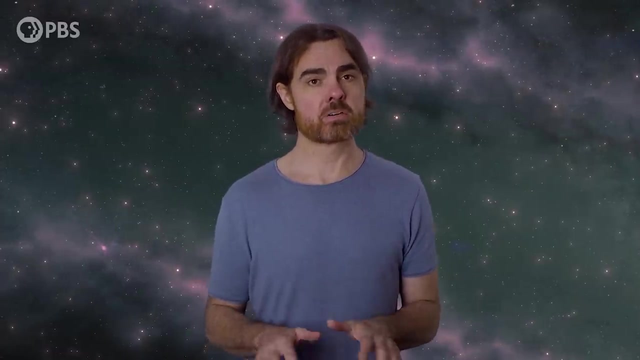 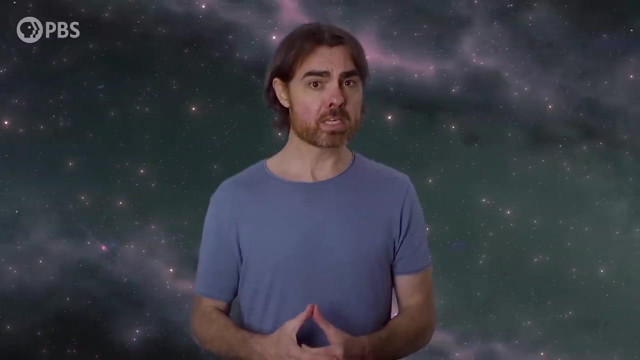 Fast forward to the early 30s. While the brand new field of quantum mechanics could describe the behavior of electrons, nuclear processes remained mysterious. Enrico Fermi made the first attempt at a full quantum description of beta decay with his 4-Fermion interaction. Basically, he tried to model this as a direct interaction in which all 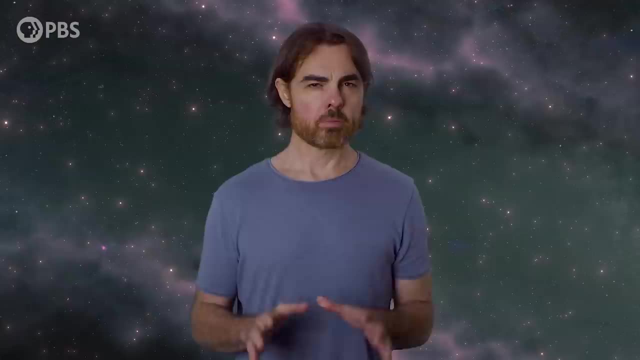 four fermion particles literally touch. So an ingoing neutron is directly converted into an outgoing proton, electron and neutrino, with all the conservation laws satisfied. Fermi was motivated by the apparently extremely short range of that interaction, And that short range is what earned. 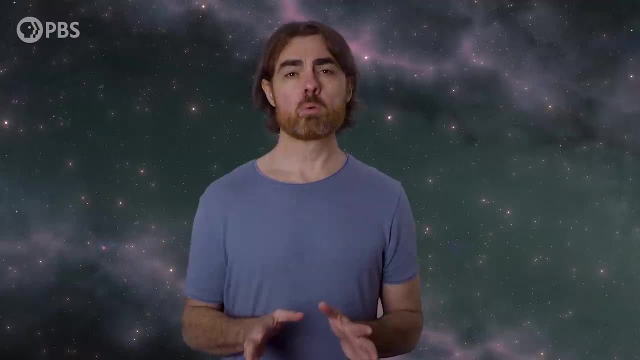 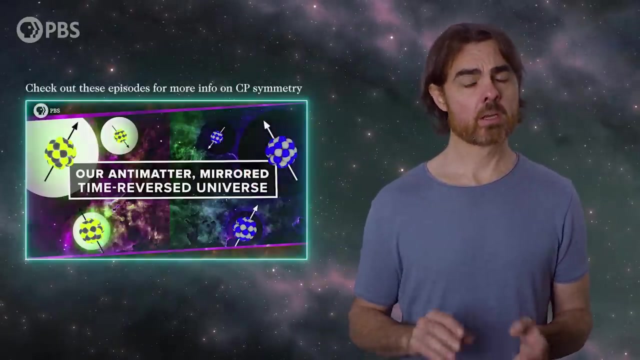 it the name, the weak interaction. But Fermi's model only worked at low energies and neither it or its successors explain why the weak interaction violates charge parity symmetry. Meanwhile there was a very different effort to explain electromagnetism that was enjoying much. 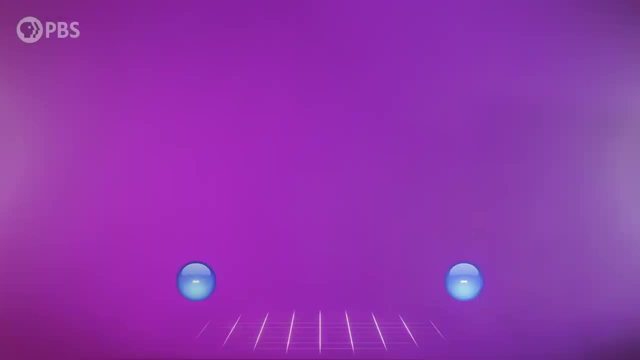 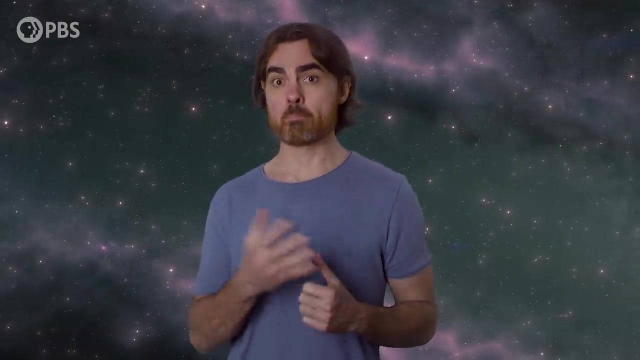 more success. That effort was quantum electrodynamics, in which charged particles interact not by touching but via a mediating particle that transmits the force, The midichlorian, I mean the photon. By the way, force-mediating particles are bosons as opposed to the fermions. 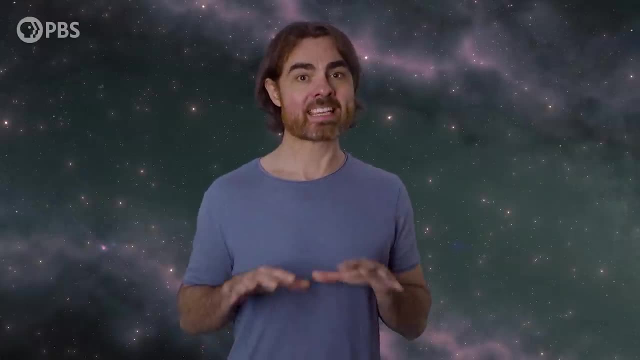 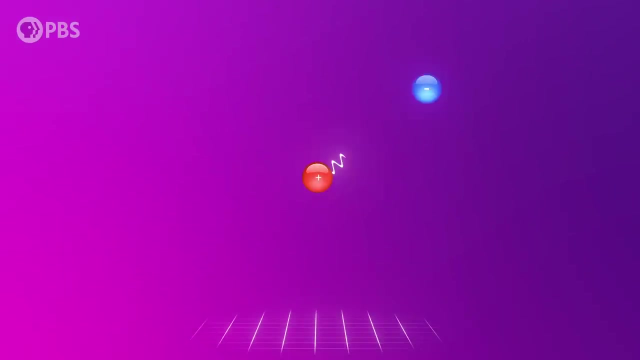 that make up matter. QED is what we call a gauge theory. Its force-carrying fields and particles arise from the symmetries of the quantum equations of motion, And we'll come back to that. In 1957, Julian Schwinger proposed a set of force-mediating gauge bosons for the weak interaction. 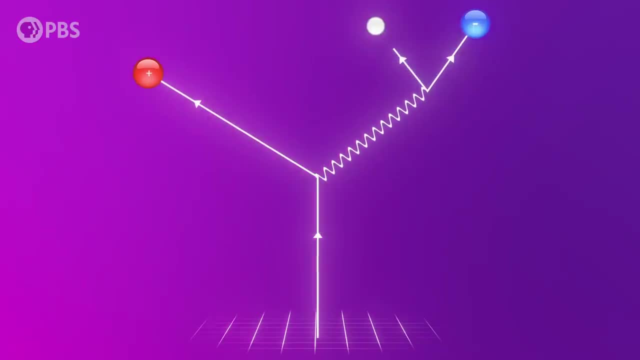 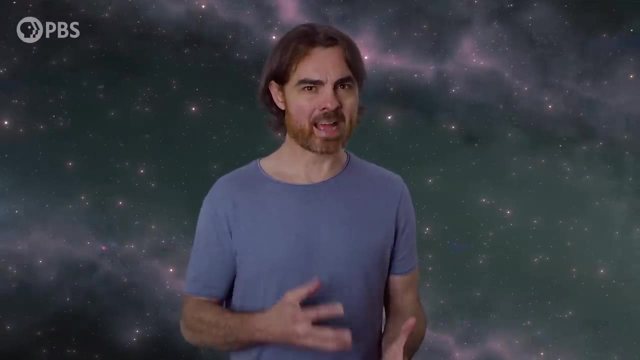 Given that the weak interaction could change a neutral particle into a pair of charged particles, this mediating particle must itself be charged. This was an early hint that somehow the electromagnetic force, which acts as a mediating particle, could change the force of a neutral. 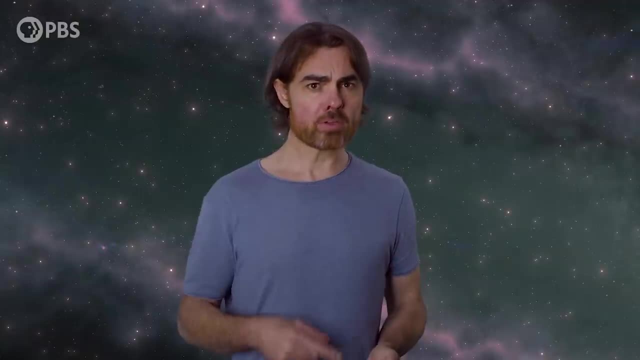 particle into a pair of charged particles. This was an early hint that somehow the electromagnetic force, which acts on charged particles, was playing a role here, although the involvement of the neutron and neutrino meant it couldn't be entirely electromagnetism. Not only that, 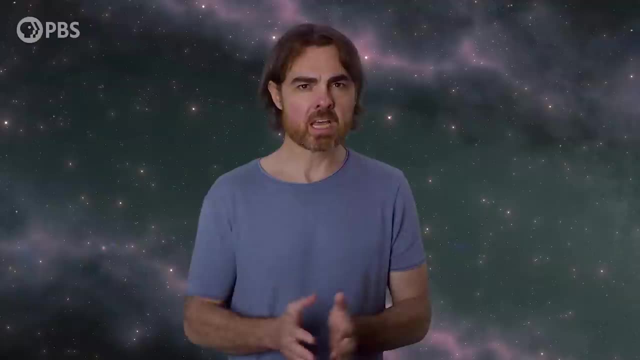 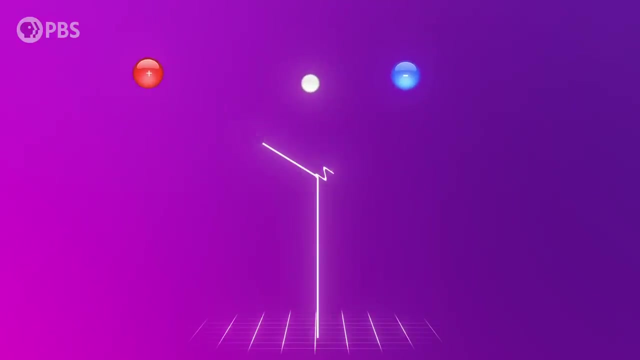 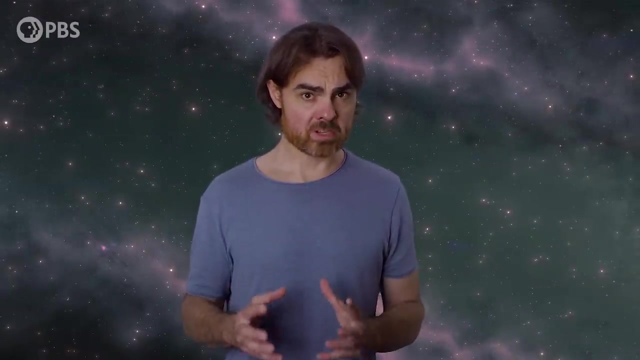 but experiments at the time indicated that if they existed, these new weak bosons, W-bosons, had to have mass due to the short-range nature of the interaction. And quite a lot of mass, in fact. The short-range nature of those forces that have massive force carriers is usually attributed to 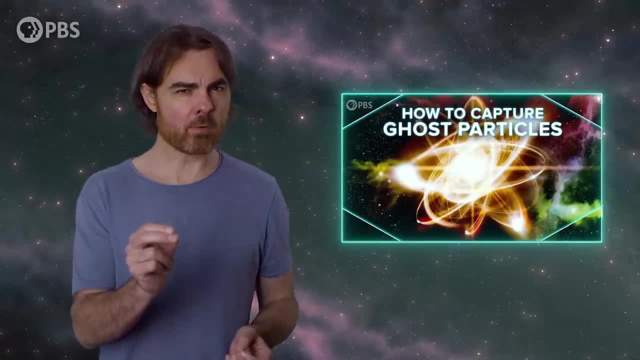 the energy of the interaction. The energy of the interaction is the energy of the interaction. The energy of the interaction is the energy of the interaction. The energy of the interaction is the energy time uncertainty relation, and we've presented it that way previously, though, as we'll discuss. 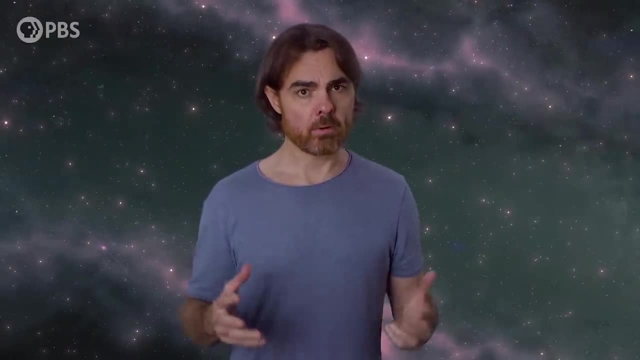 in a future episode. that is not the full story. Anyway, this new gauge theory of the weak interaction seemed to be OK with parity violation, and it wasn't only accurate at low energies. So problem solved, Easy peasy right? Well, not even close. 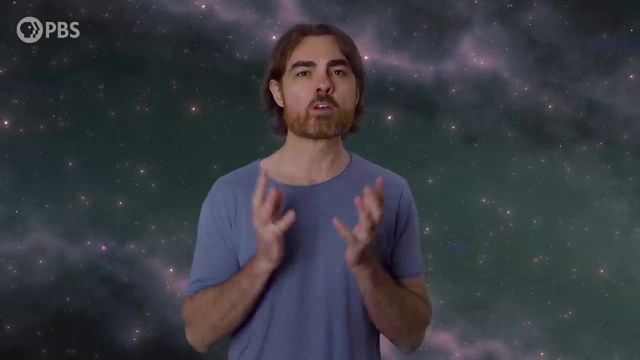 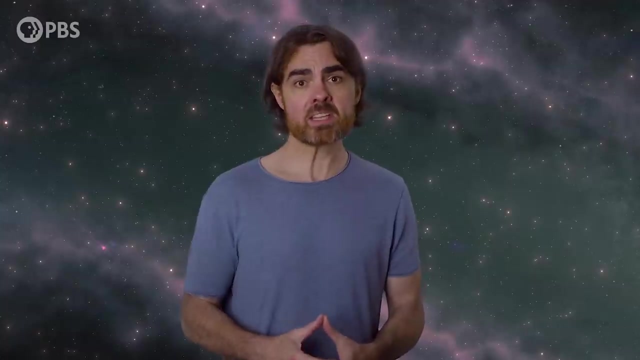 That requirement of the W-bosons having mass was an enormous theoretical headache. Gauge bosons should not have mass Ever, At least assuming that the symmetries of the gauge theory remain intact. But, as we'll see, the simple requirement that the weak force was mediated. 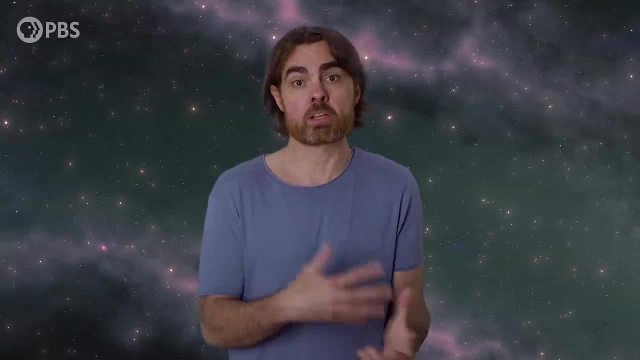 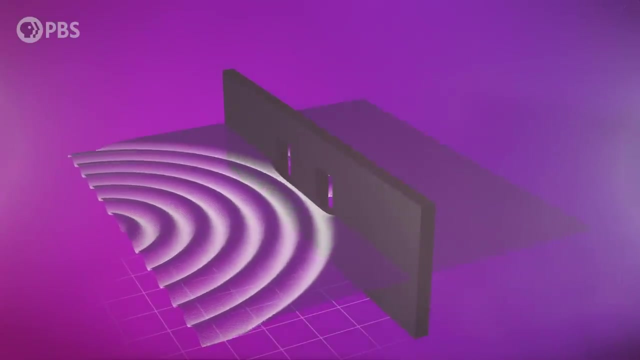 by massive particles ultimately unified the weak force with electromagnetism and revealed the existence of the Higgs particle. To get to all of this, we need to do a quick recap of what a gauge theory actually is. Let's try an example In quantum mechanics: the wave. 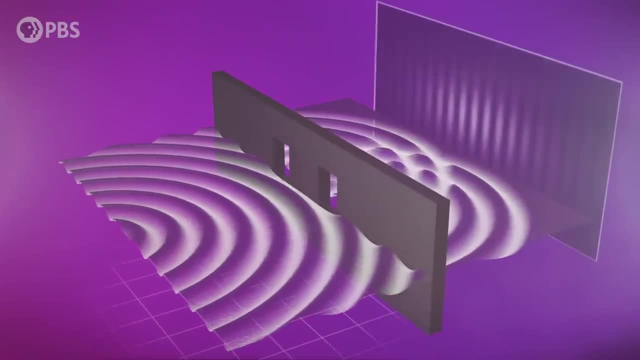 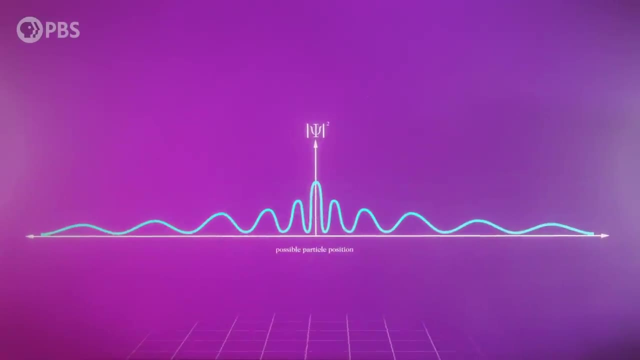 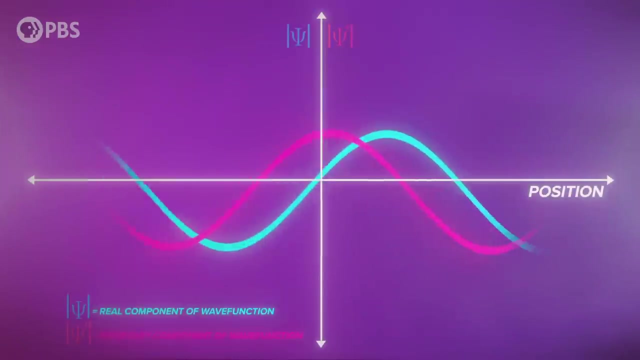 function determines the probabilities of certain outcomes being measured for observables like particle position and momentum Quantum. mechanical equations of motion, like the Schrodinger equation, describe how the wave function evolves through space and time. Like all waves, the wave function has a phase. the current position of peaks and troughs. 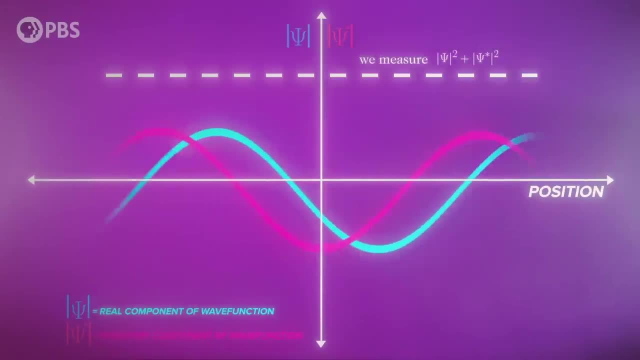 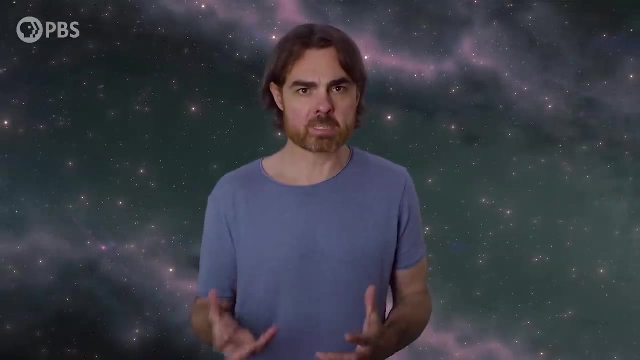 But that phase should be totally unobservable by any experiment. Phase is what we call a degree of freedom, because it should be possible to change it however you like at any point in space and still get the same physical observables. For that to be the case, we need to add some stuff. 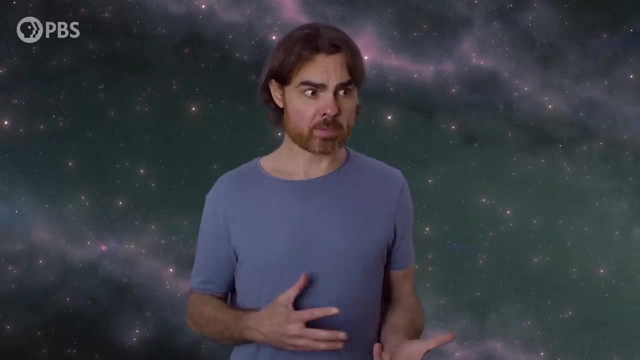 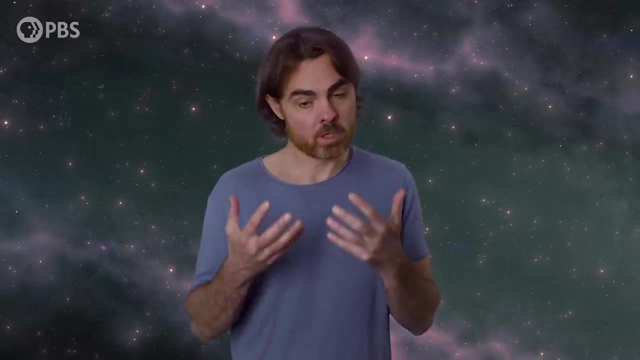 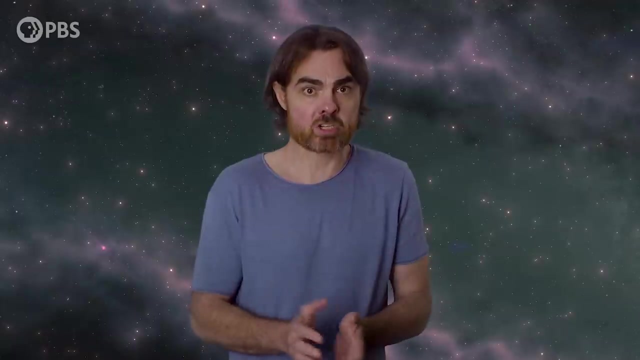 to the Schrodinger equation. That stuff turns out to describe the electromagnetic field. And when we quantize that field, when we let it oscillate with discrete packets of energy, we get the photon. So there we go. We insisted on a symmetry, that the Schrodinger equation is invariant to changes. 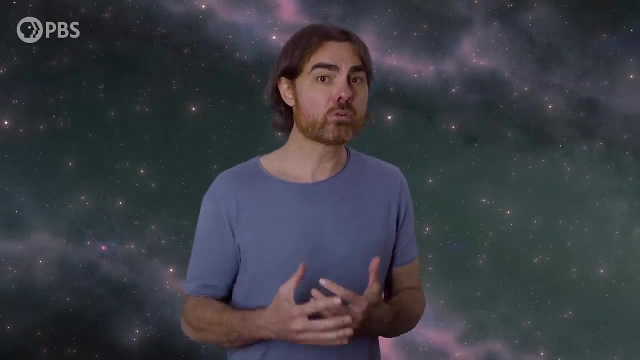 in the local phase of the wave function. that resulted in a new quantum field and a corresponding particle. So that is gauge theory in a nutshell. It explains a force by imposing symmetries on the equations of motion. Actually, a visual representation would really help here. 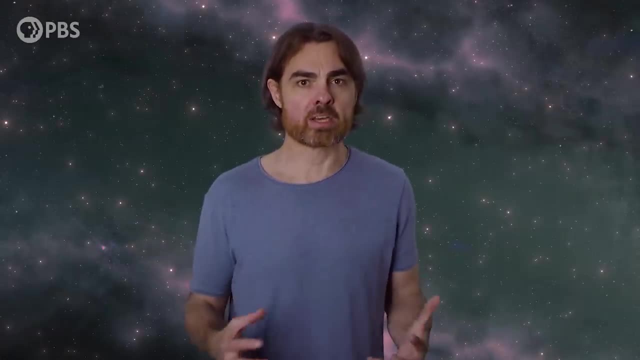 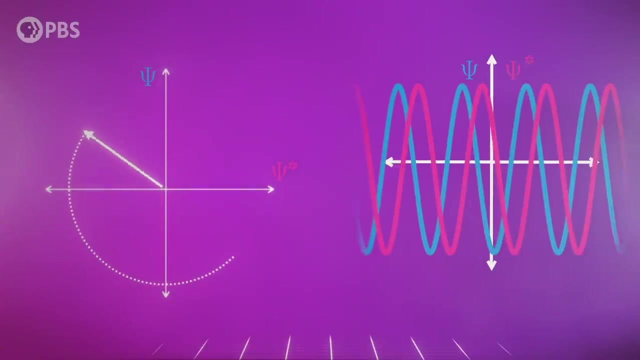 We said that at each point in space the physics shouldn't change. when we shift both the real and complex parts of the wave function by some amount, We shift the phase A process, which leaves the magnitude of the wave function unchanged. This is equivalent to considering a complex 2D vector. 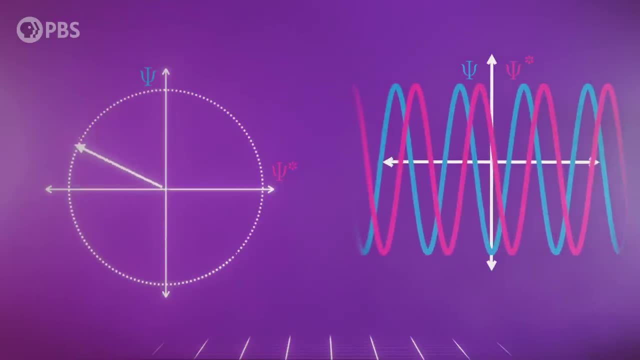 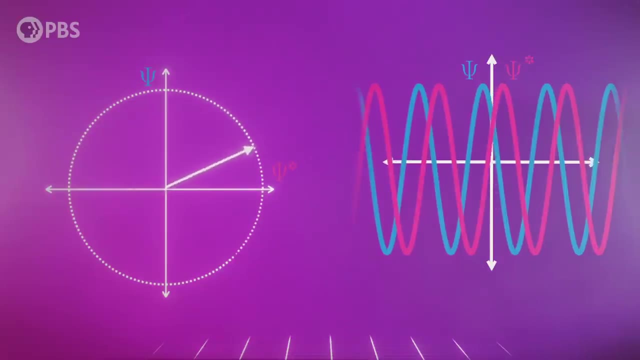 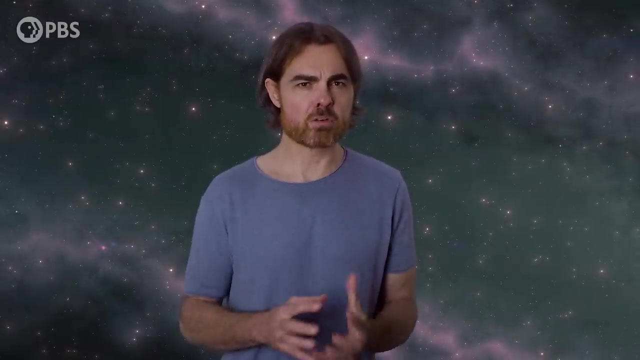 Where the axes are the real and imaginary components which we can rotate but not stretch or shrink. The length of the vector is the magnitude of the wave function and the rotation amount is our local phase shift. The collection of transformations which describe rotations of 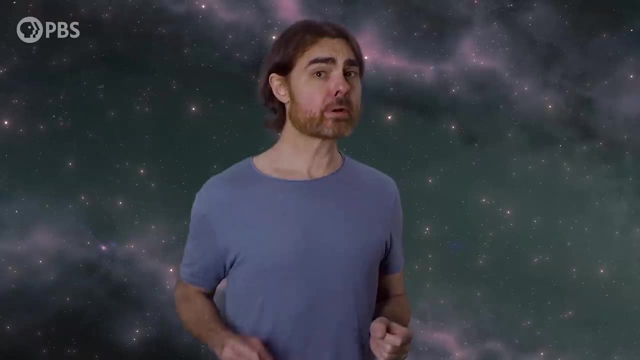 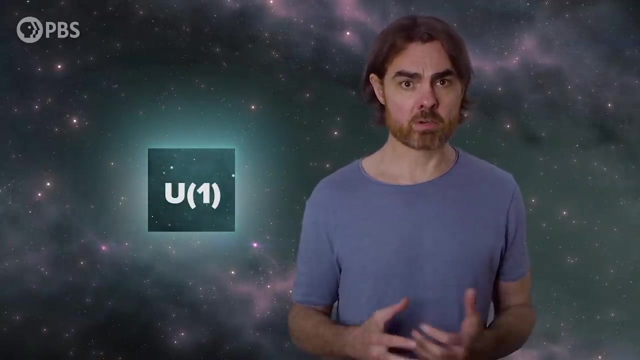 2D vectors are members of something called the unitary group of size 1, written U1.. The U stands for unitary and tells us that the elements of the group preserve vectors. The U1 just means the symmetry transformations act on states which can be completely represented. 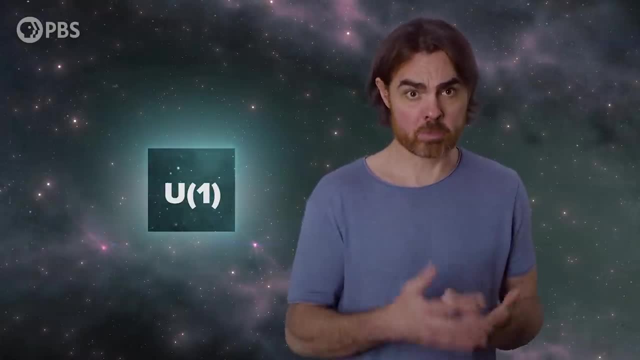 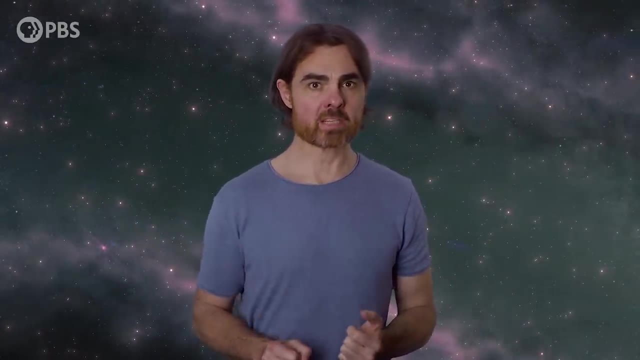 by just one function, like our single wave function from the Schrodinger equation. Imposing this U1 symmetry on our equations of motion led us to something very real and physical: electromagnetism. So it makes sense to see what other symmetries do. 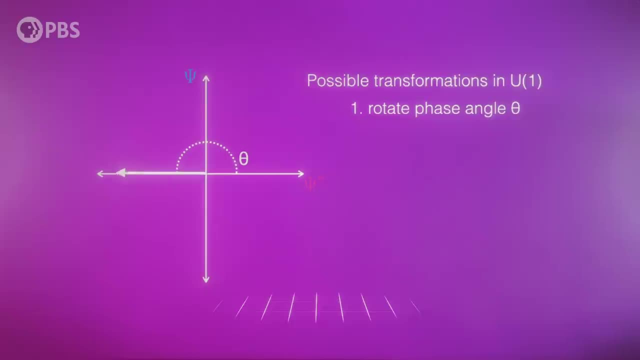 There, the single 2D vector could only change in its angle, its phase. It had one degree of freedom corresponding to a gauge field with a single mode, the electromagnetic field and its photon. In SU, each individual vector can change length, rotate and be reflected. 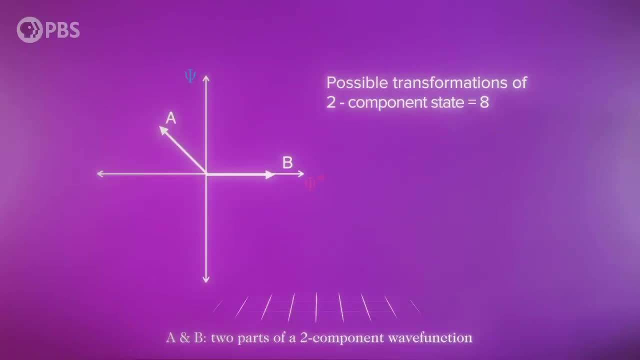 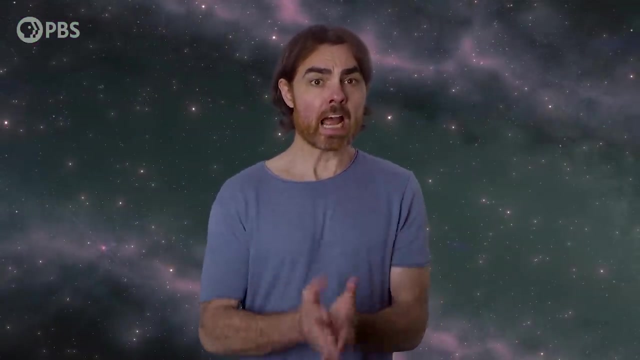 overall 8 degrees of freedom. But if we require this transformation to now respect SU symmetry, for example requiring unitarity, we knock out 5 degrees of freedom, leaving us with only 3.. If we require our equations of motion to respect SU, we have to introduce a new. 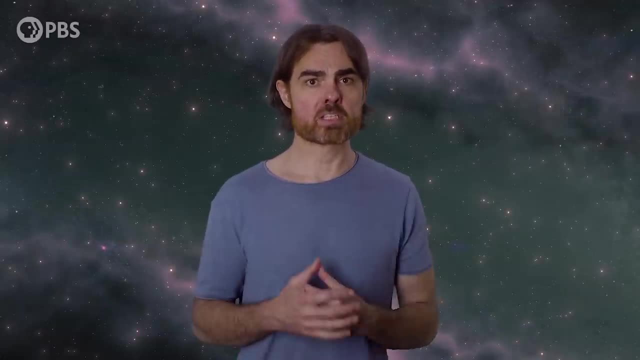 field with 3 degrees of freedom. Quantizing this field gives us 3 bosons which are almost exactly what we need to make a gauge theory of the weak field work, Almost The fields and corresponding particles produced by the pure symmetries we described. 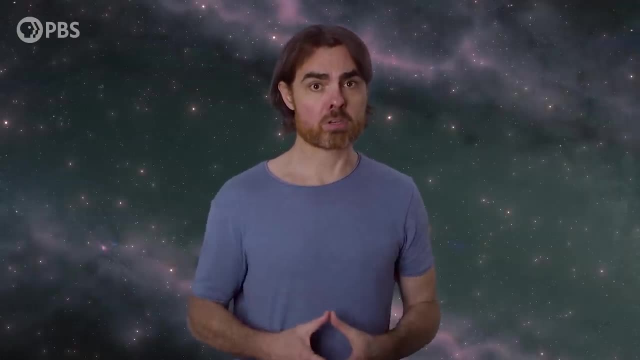 are fundamentally massless. The bosons of the version of SU that I just described are simple light-speed oscillations in their fields, just like photons, But the bosons of the weak force have to have mass. So is this a bust? Well, maybe, But the whole gauge field thing seemed so promising. 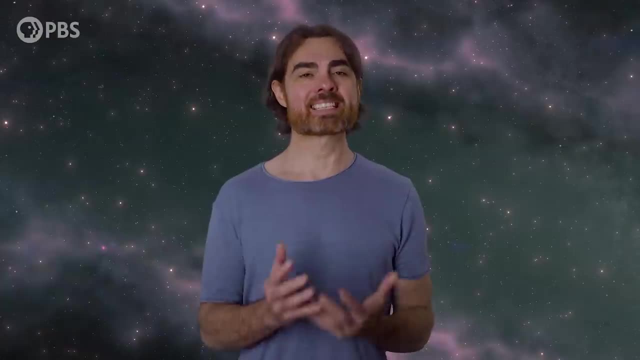 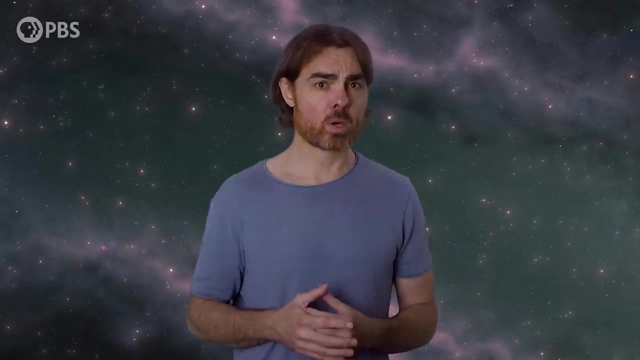 So it's worth asking: how can we give mass to something that seems fundamentally massless? The perfect masslessness of these gauge fields and bosons is a direct consequence of the perfect symmetries from which they come. Adding mass screws up those symmetries. For example, adding mass to a 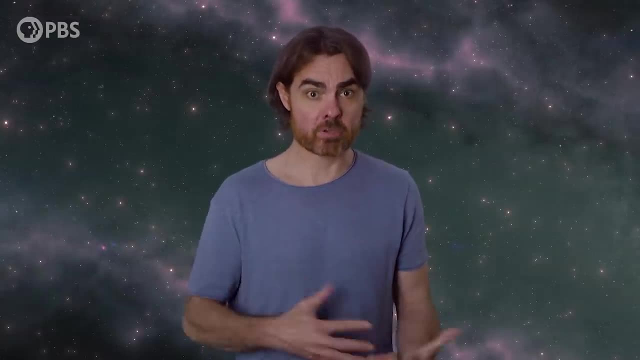 random boson means adding an extra term to the electromagnetic field stuff in the Schrodinger equation so that it would no longer be invariant to local phase shifts. In order for the weak force bosons to have mass, we have to willingly break the symmetry that gave us them in the first place. But wouldn't that mean throwing away the core idea that gave us the weak field? Not necessarily. It's possible for the equations of motion describing a system symmetry to not care about changes in some property but at the same time for the state of the system those equations describe to not have the same symmetry. 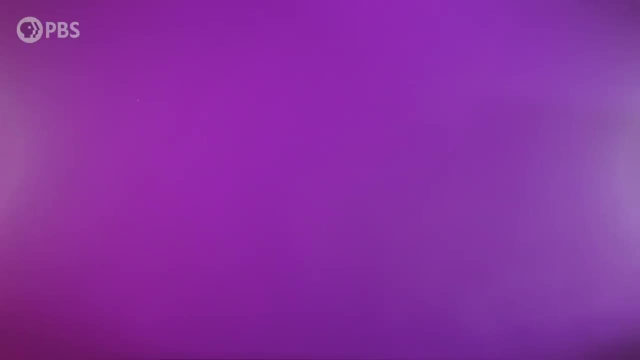 That sounds counter-intuitive. so let me give you an example. Consider a magnetic material made up of many little magnetic dipoles, like little bar magnets, that can point in different directions. The equations of motion governing the overall magnetization of this material aren't encoded. 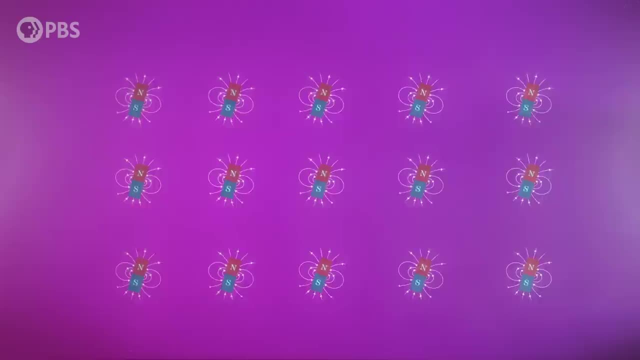 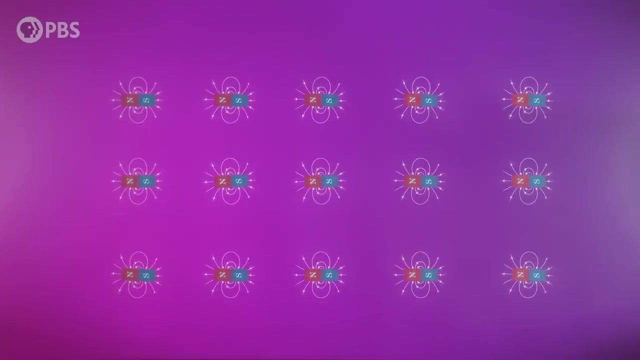 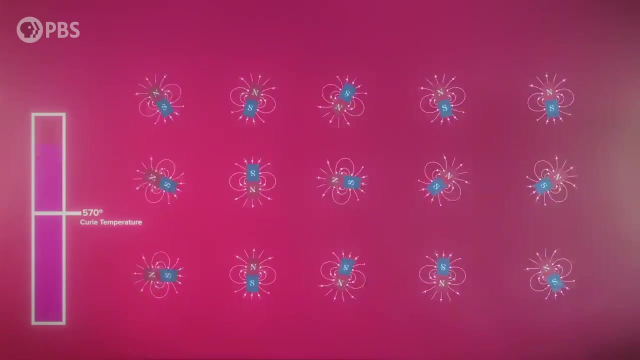 with some special direction, the whole system could be rotated and nothing would change. This represents the symmetry in our equations. But the individual magnetic particles interact with each other. They want to align with their neighbors At high enough temperatures above the Curie temperature, in this case, thermal energy causes. 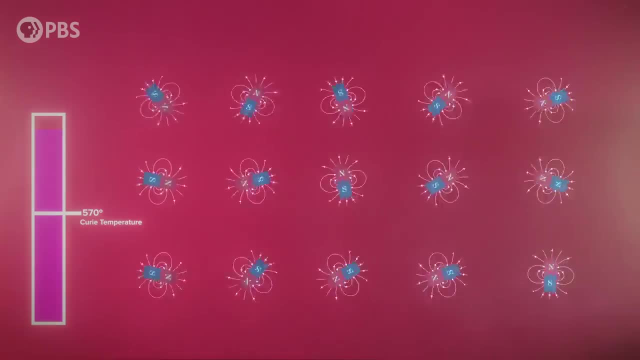 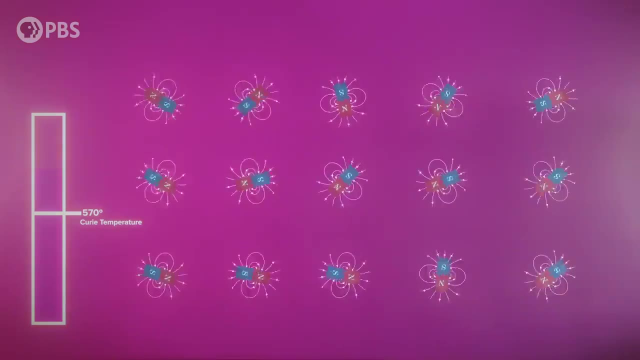 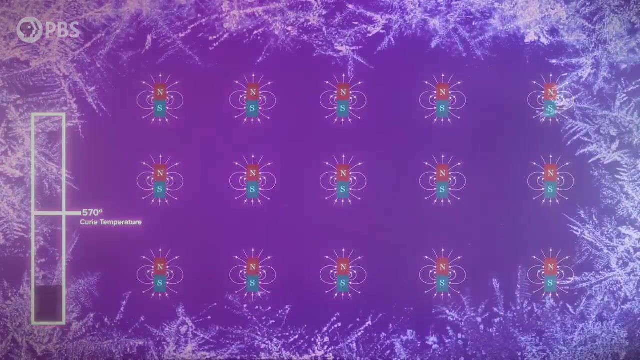 the particles to rotate randomly, so the overall magnetization of the material is random. However, if we cool the material down, the interactions between magnetic particles can start to come into play. They align with each other. If we cool the system enough, all particles get frozen into one aligned state. 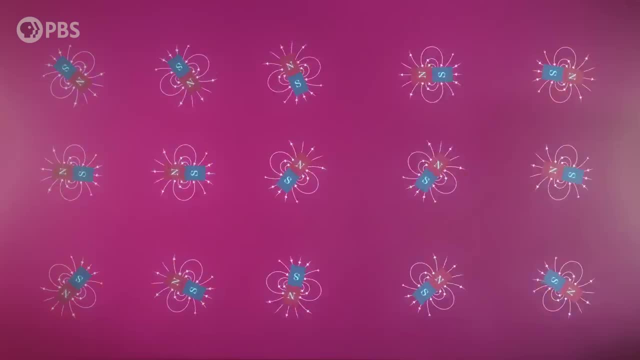 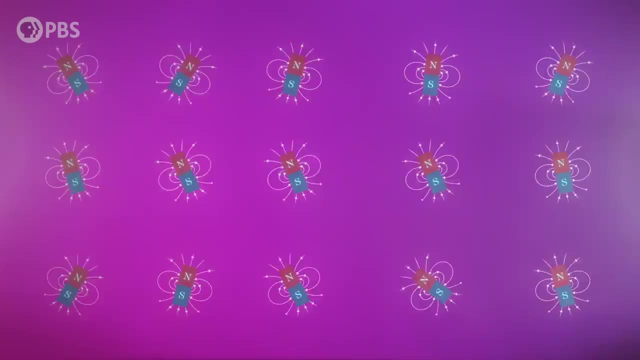 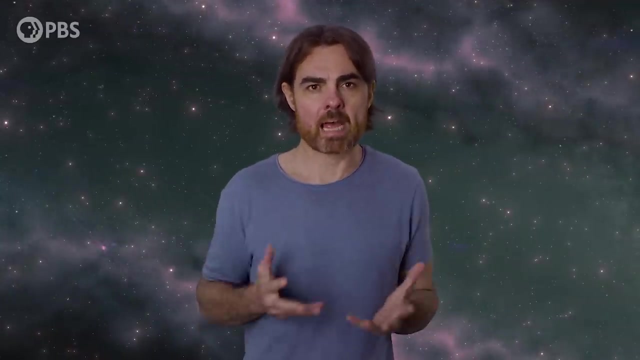 This is a state of broken symmetry. Even though the equations of motion say one direction is not preferred to any other, the ground state has randomly picked out a single direction. We call this spontaneous symmetry breaking. So what if something similar is happening with the field? that gives us the weak force. 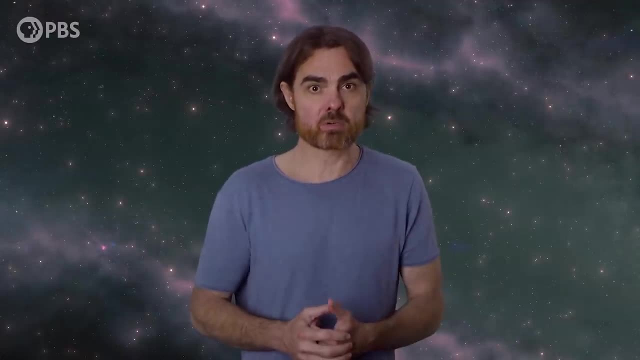 Perhaps the equations of motion respect the symmetries that give us the necessary gauge field, but the physical system, the field itself, evolves into a state which no longer respects those symmetries. That could lead to our force carriers having mass. This has been an analogy-heavy episode. 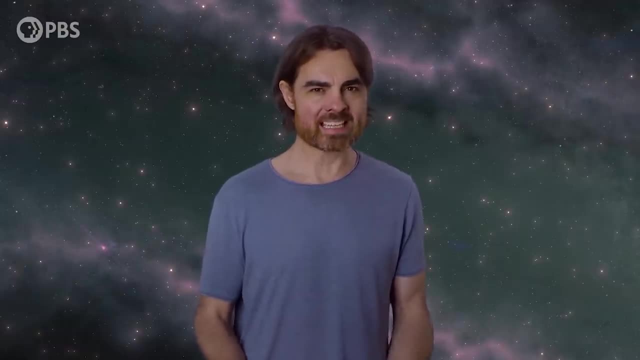 Spinning vectors, magnetic materials. But what specifically is happening with the weak field? What is this symmetry And what causes it to break? Or remember that I said that the weak interaction somehow seems to involve electromagnetism? That's another clue. 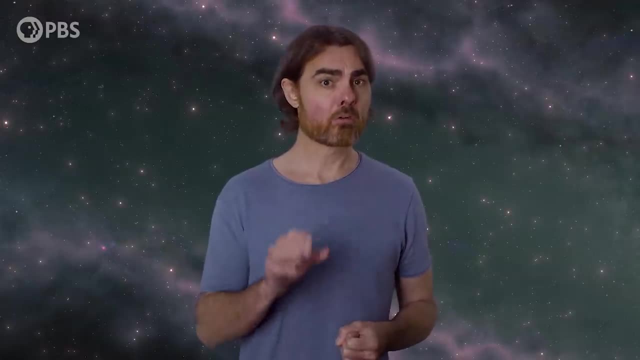 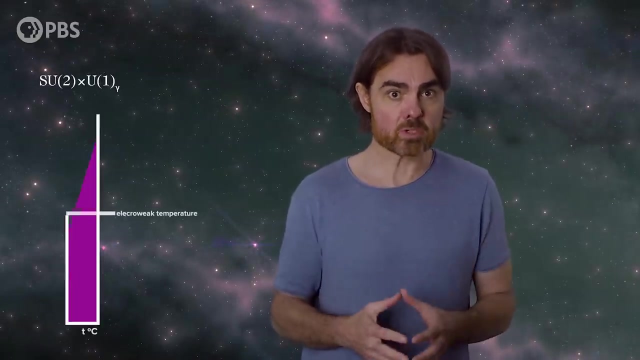 It turns out that both the weak force and electromagnetism come from the breaking of a larger symmetry group. And actually that larger symmetry group is just the combination of our U1 and SU2 symmetries. The combined SU2 cross SU1 symmetry is the electroweak field and it has four massless. 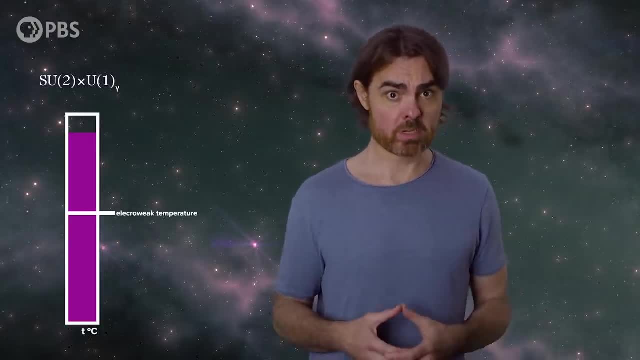 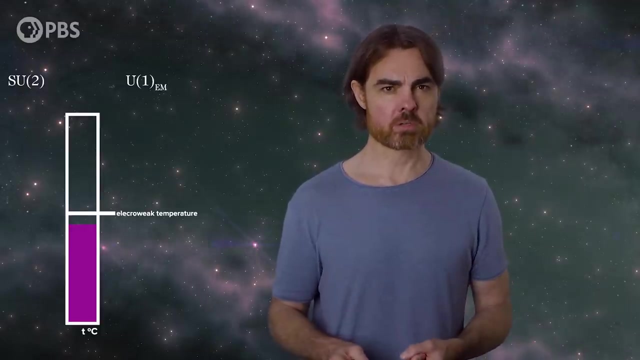 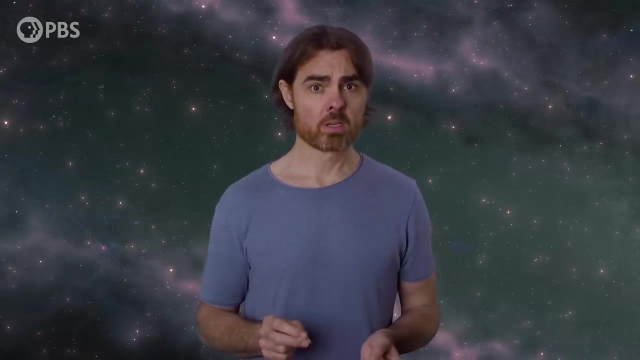 bosons, Like a well-behaved symmetry should, But at low temperatures this symmetry is spontaneously broken, leaving an independent, massless S1 field for the photon and a massive broken SU2 field that gives the massive weak force bosons. By the way, by low temperature I mean anything below around 10 to the power of 15 kelvin. 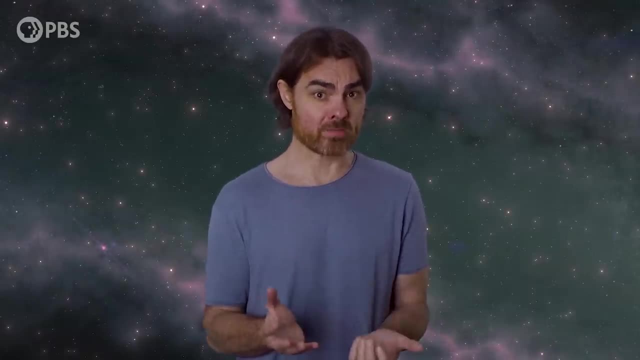 The entire universe was that hot when it was less than a trillionth of a second old. Back then, electromagnetism and photons and the weak force didn't exist And the weak force didn't exist. And the weak force didn't exist. 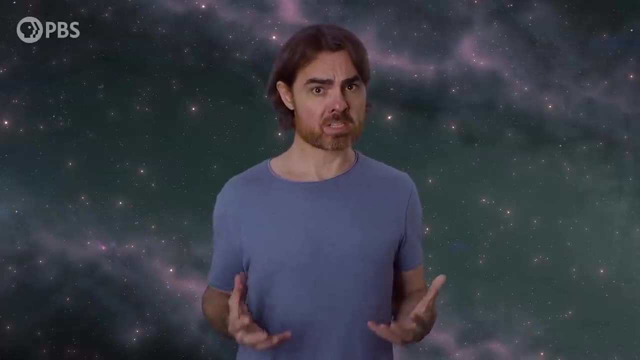 This was the electroweak error, And we can also produce these conditions in our particle accelerators, And in fact we've verified the whole electroweak thing with fantastic precision. Let's take a second to remember how we got here. 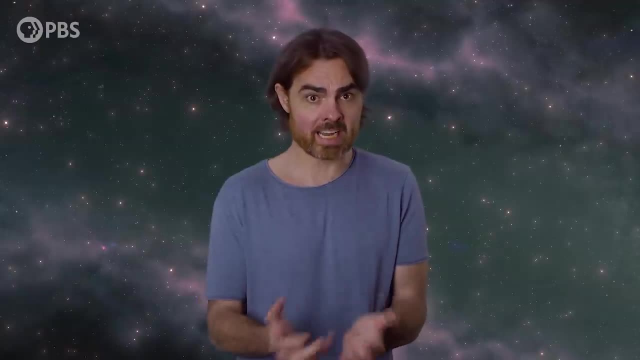 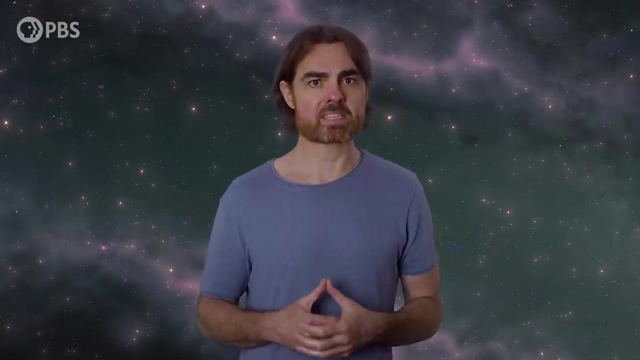 We just asked what would happen if the equations of motion governing nature had certain symmetries. The very existence of those symmetries requires a family of fields and particles that we now observe in nature. But to really make this work, to give the weak force, bosons, their mass, we have to conclude. 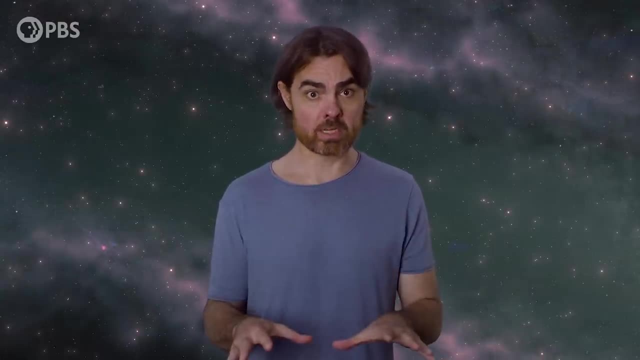 that really, these fields, these symmetries, are ultimately unified And then broken, As we'll see soon, by the Higgs field. But it doesn't stop there. The electroweak unification sets us on this grand quest to find deeper symmetries. that 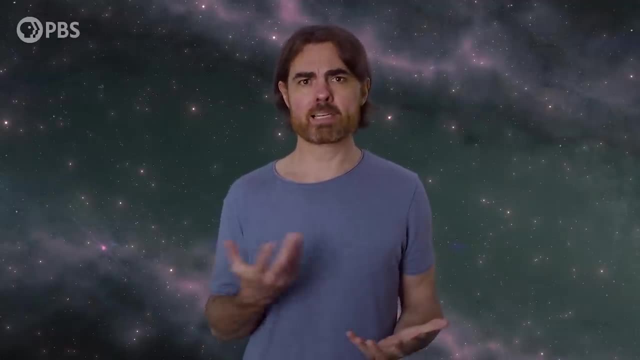 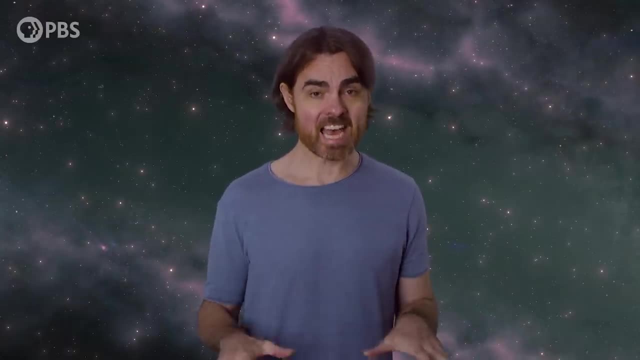 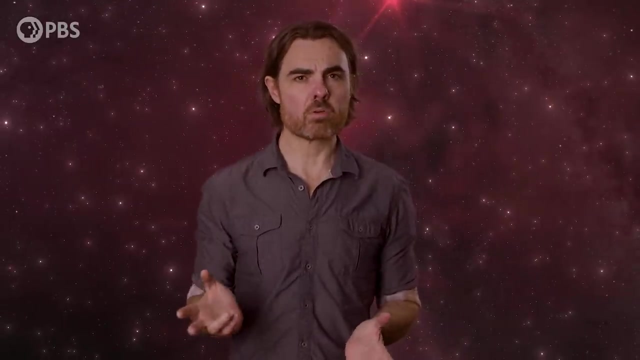 U1 cross F2.. U1 cross F2.. And from which arises the fantastically rich palette of particles and the complexity that they enable: Inevitable consequences from the broken symmetries of spacetime. Last time we talked about singularity theorems and how they show that the singularities at 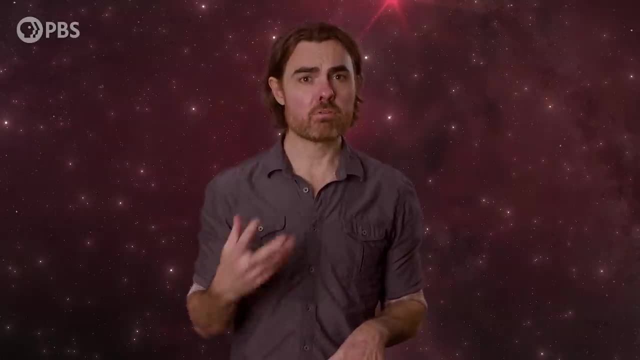 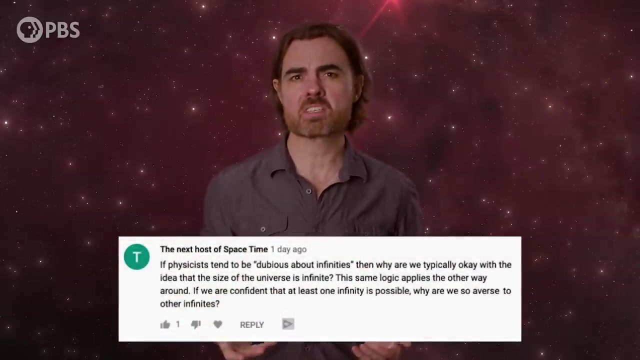 the heart of the black hole and at the big bang are inevitable if you follow only general relativity. Let's see what you had to say. The next host of spacetime asked us: If physicists tend to be dubious about infinities, why are we then typically okay with the size? of the universe being infinite. Well, I think this is a fair question, But there are different types of infinities and some are seen as worse than others. The singularity type is considered a bad one. That's when some property blows up to infinite values, like the density or curvature at the 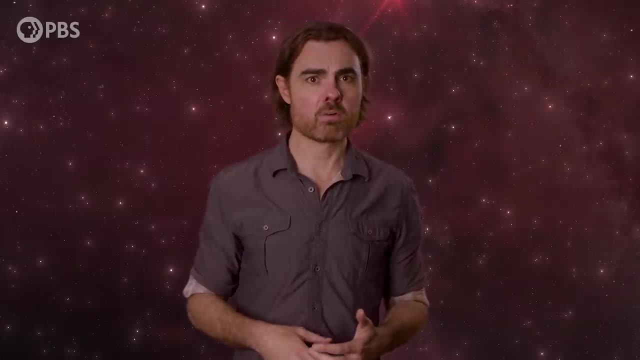 center of a black hole. In the case of the black hole singularity, or the singularity of the big bang, it's bad because it causes irreconciled conflicts with the universe. Quantum theory, in this case An infinite universe, doesn't have the same problem and I guess it's often accepted. because it's actually not much more philosophically satisfying to propose a finite universe. You can as well ask why does the universe stop where it does, as you can ask why does it go on forever, But hold onto your unease. These are the intuitions that can lead us forward. 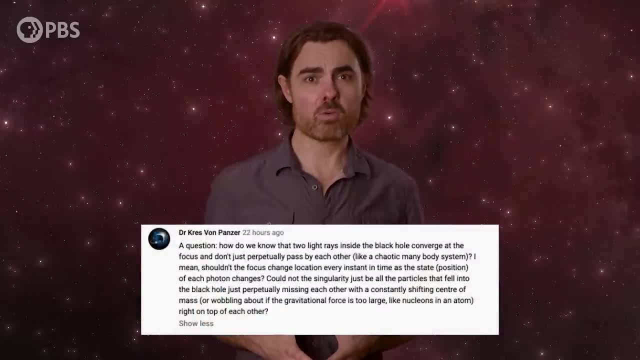 Dr Kles von Panzer asks how we know that two universes are infinite. He says that the universe is infinite. He says that the universe is infinite. He says that two light rays inside a black hole converge and don't just perpetually pass. 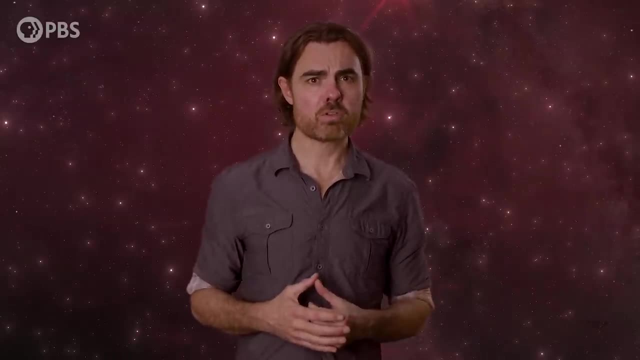 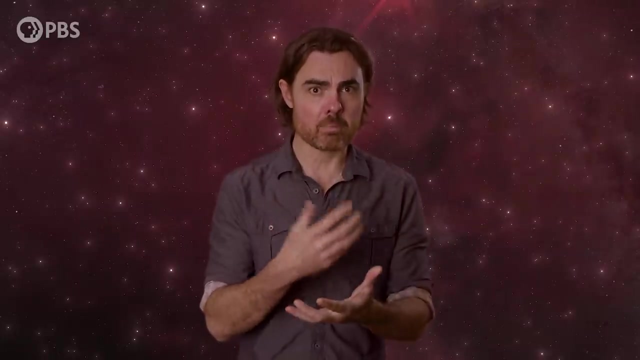 each other. Well, really, this is the core of Penrose's proof. He showed that at least some light rays- null geodesics- that start out parallel from any trapped surface must converge in any positively curved spacetime. Not all of them necessarily converge, but you only need some to do so to get the singularity. 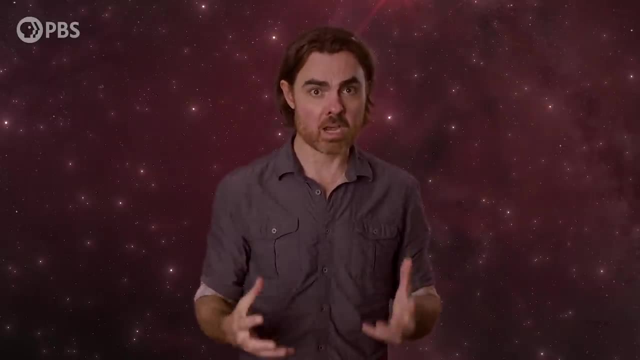 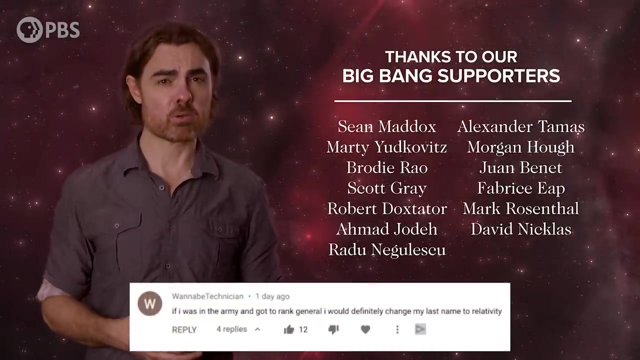 In the case of the perfectly spherically symmetric inside of a Schwarzschild black hole, all of the geodesics do indeed converge. He says that the universe is infinite- Awesome proof. we have now A wannabe technician there says that if they became a general in the army, they would definitely